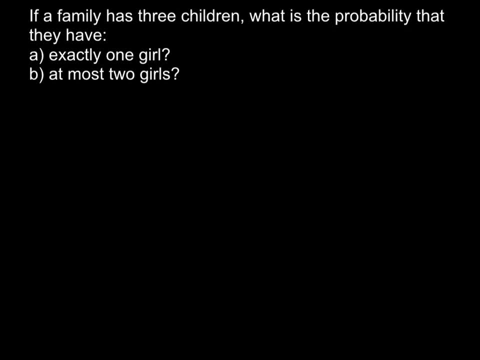 variant can be when the family would have all three children boys, So this would be boy, boy and boy. Another variant can be when there can be two boys and one girl, And this can be boy, boy and girl. Another variant can be boy. 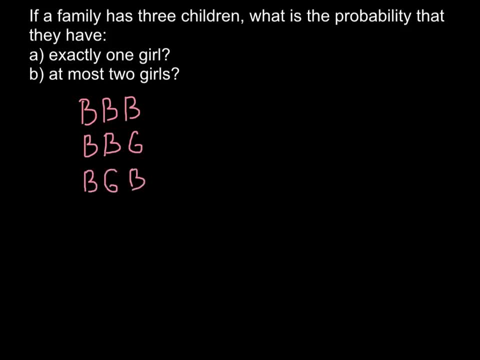 girl, boy, And another variant when the first child is girl and then boy and boy. Also, this family may have two children, that is, girls and one child that is boy. So variants possible here: girl, girl and boy. Another variant can be girl, boy and girl. And the last variant can be boy, boy and girl. 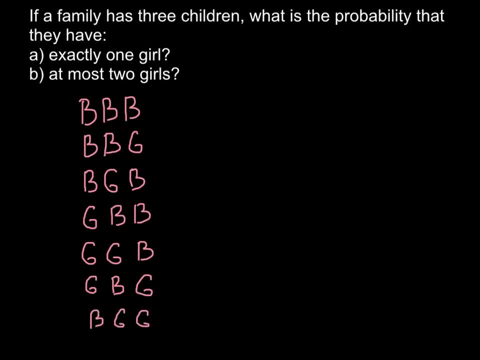 And girl and girl. And also family may have three children, that is, girls. So this would be girl, girl and girl. So let's count how many variants this family would have. So one, two, three, four, five, six, seven, eight, Eight variants. And now 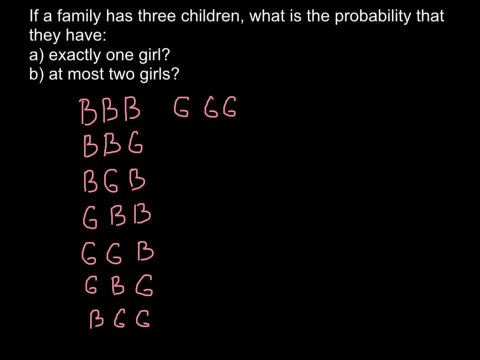